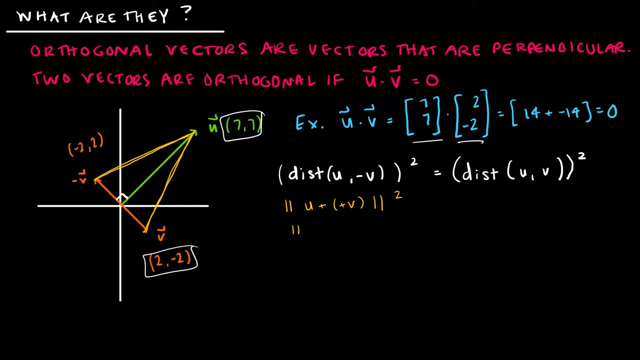 So essentially, I have find the distance of u plus v, Square it. So the distance of u plus v would be u plus v and the inner product with itself u plus v. Oops, not squared anymore, And using some of the properties that we know, I have that u with the product of u plus v. 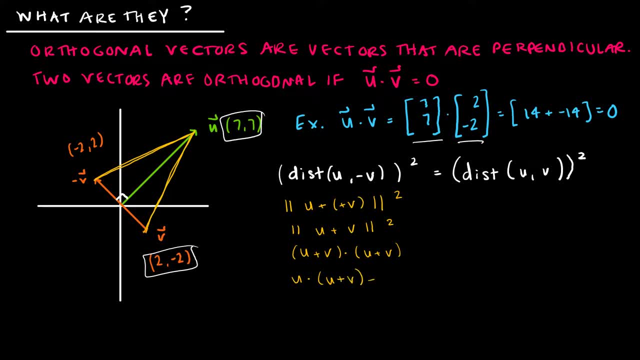 so the inner product of u with u plus v, plus v times, u plus v inner product And again doing a little bit of more of our properties, we've got u and u here so I can say u inner product of u and u. 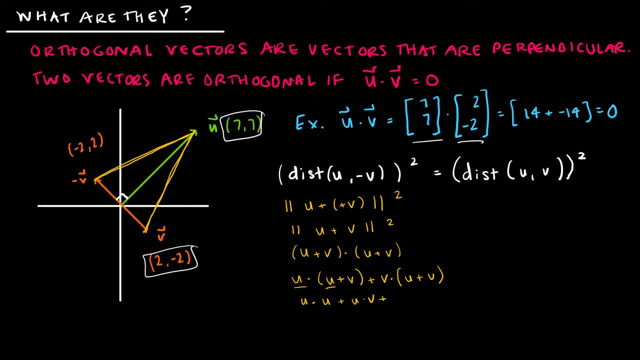 plus the inner product of u and v, plus the inner product of v and u, plus the inner product of v and v, which is essentially, which is essentially, which is essentially the length of u squared plus the length of v squared plus 2, u inner product v. 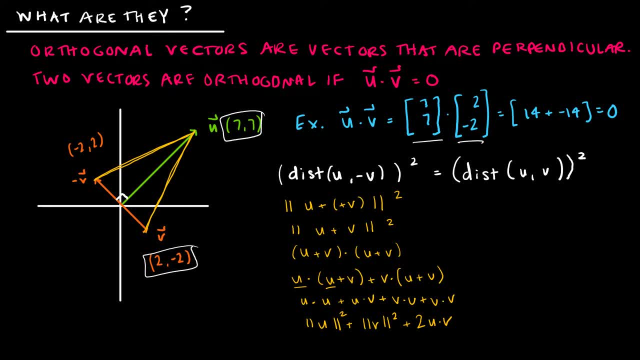 If I do the exact same thing on the other side. so I'm going to be doing similar calculations over here. This is going to be u minus v, Because that's how we compute the distance. And then that means, and then again, u oops, u minus v. 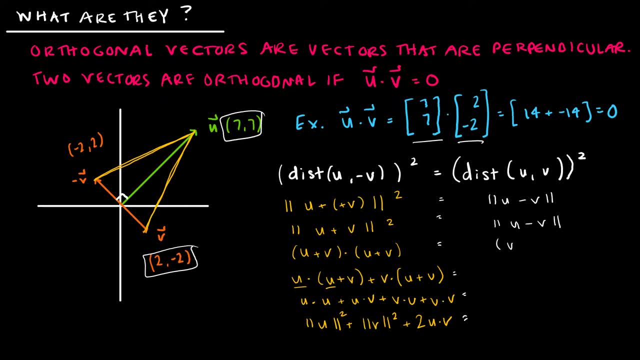 I didn't do anything on that step. So this is u minus v product u minus v. Sorry, my v's and u's are starting to look a little bit alike. And then again doing that same, using those same theorems, using those same properties. 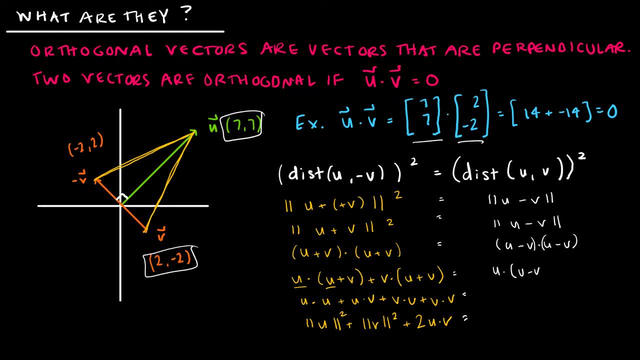 I can say u times u minus v, I'm sorry, u inner product of u minus v, plus I'm sorry, minus v, and then inner product of u minus v, And we can see that this is very, very similar. 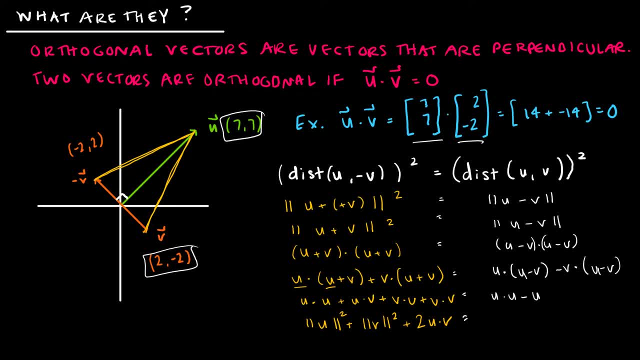 So this is u with the inner product of u minus u, with the inner product of v minus v. inner product u minus, or sorry, plus v. inner product v product v. And so, as we can see, what's happening is, I have the length of u squared plus the length. 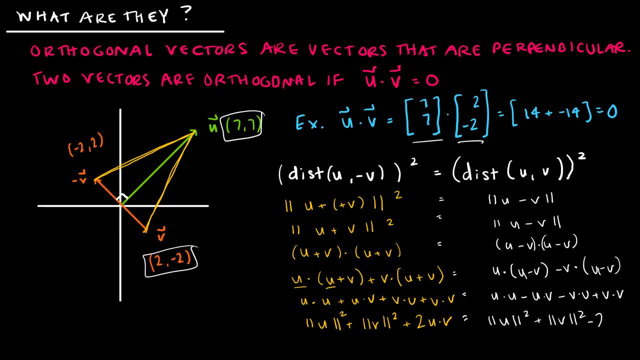 of v squared, and this time I have minus 2u inner product v, And so, essentially, what we're saying is for these distances to be the same. these obviously are the same. these obviously are the same. we need 2u inner product v to be equal to negative 2u inner product v, And the only way 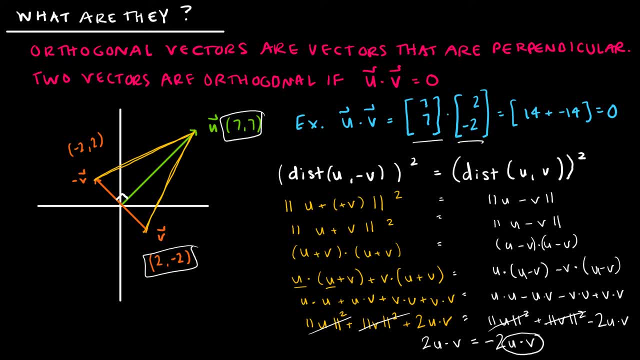 that that's going to happen is if uv is 0, because 2 times something is not going to equal negative 2 times something unless that something is equal to 0. So that's where this comes from. So hopefully that helps you to understand, just a. 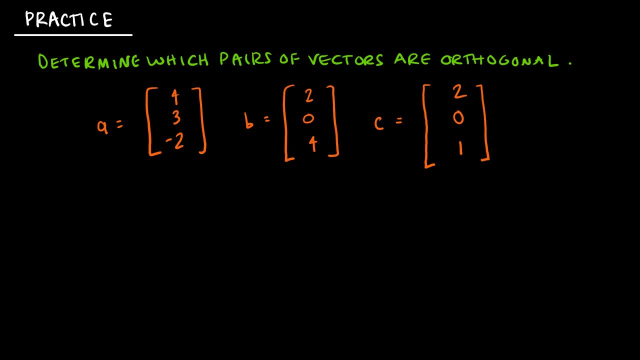 little bit more about what's going on here. So let's try this question. We're looking for which pairs of vectors are orthogonal And again, when we're doing this, all we're doing is finding the inner product. So I'm going to take 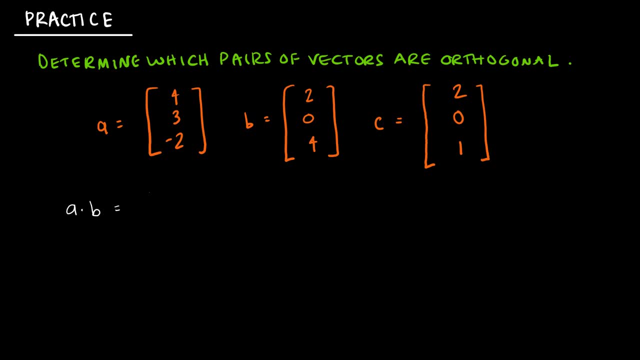 a, b and determine the inner product. So in this case that would be 4 times 2 plus 3 times 0, plus negative 2 times 4, because again that inner product just says: multiply corresponding parts. You can certainly turn it into the transpose if you want. 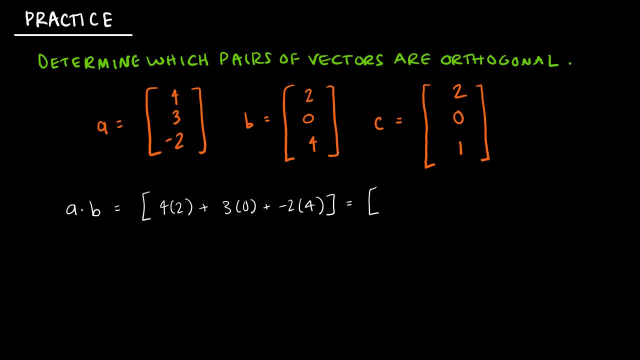 but I'm not ever going to do that. 4 times 2 is 8,. 3 times 0 is 0, negative. 2 times 4 is negative 8, and therefore my inner product is 0,. and a- b are orthogonal vectors, which means if I were to 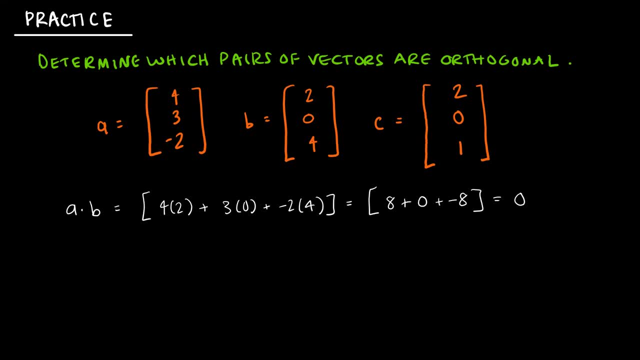 graph these, which would be more difficult, in three dimensions. but if I were to graph them, they would in fact be perpendicular. Now let's try a c. So again, a c would be 4 times 2 plus 3 times 0, plus negative, 2 times 1,.